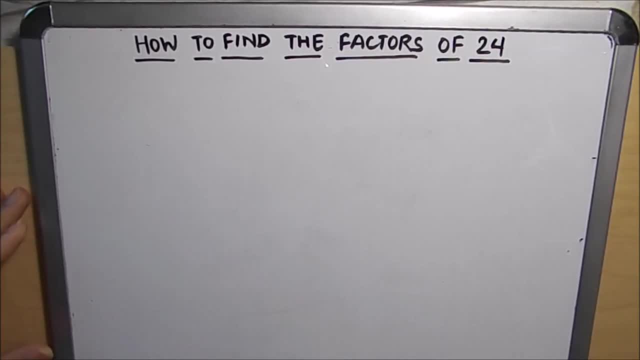 Hello viewers, in this video we are going to find the factors of 24.. So what are factors? you all must be knowing that factors are numbers which multiply to give a product or the other. definition can be: factors are numbers which divide a number fully without leaving a remainder. So let's see. 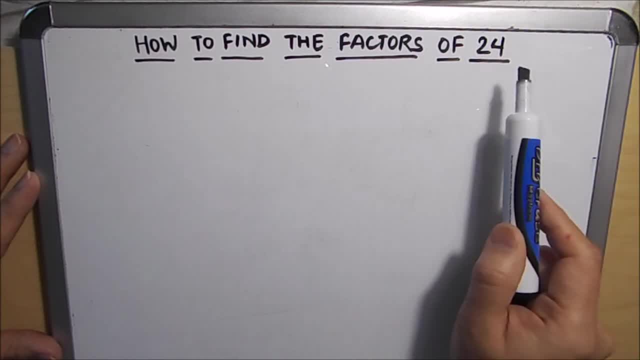 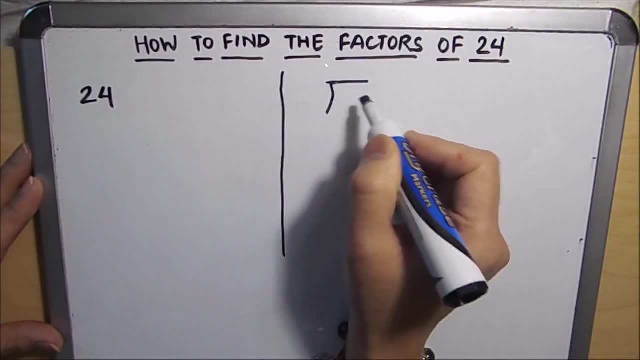 how we find the factors of any number. Here we are finding the factors of 24.. So to find the factors of 24, we'll start with number 1 here and start dividing 24 by 1.. As 1 is a factor of all. 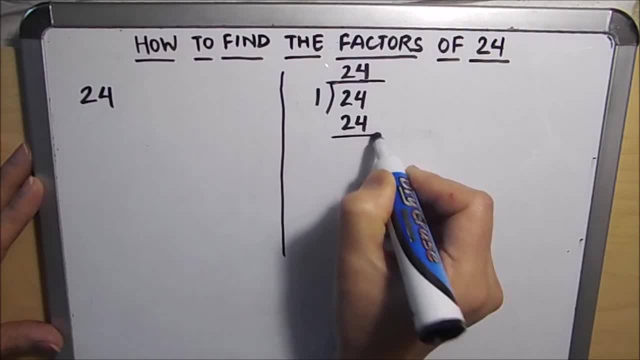 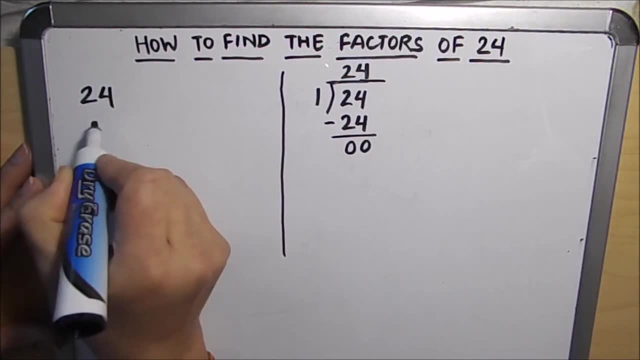 the numbers. so 1 is a factor of 24, because 1 times 24 is 24 and we are getting 0 remainder, So we will write 24 as 1 times 24.. So here from this we concluded that 1 is a factor of 24.. Next, 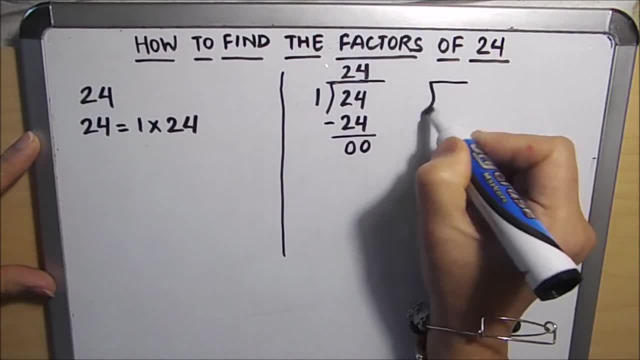 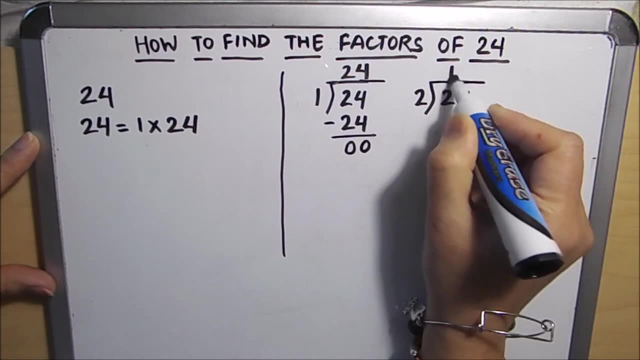 we will move to the next number, which is 2, and we will divide 24 by 2.. So 2 times 12 is 24 and we are getting 0 as a factor of 24.. So we will write 24 as 1 times 24.. So here from this we. 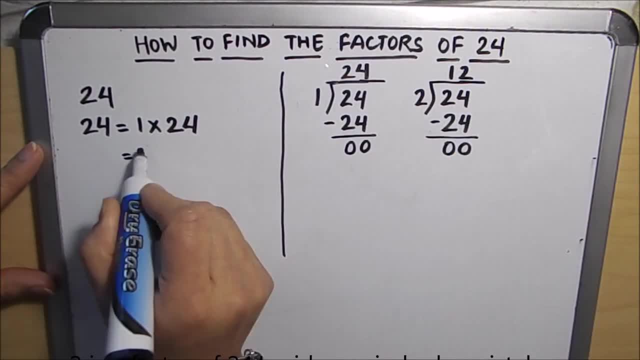 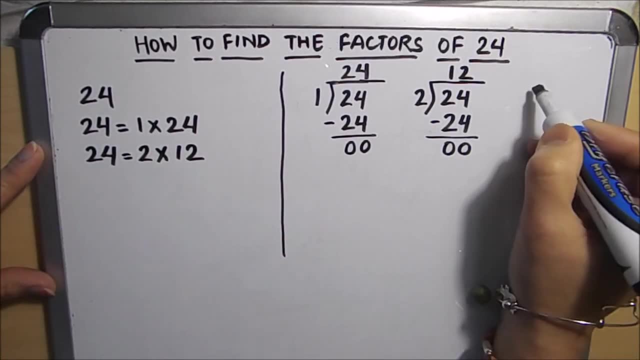 concluded that 2 is a factor of 24.. So this also concludes that 2 is remainder of 24, and we can write 24 as 2 times 12.. Next number: we have taken 1, 2. now we will move to number 3 and we will. 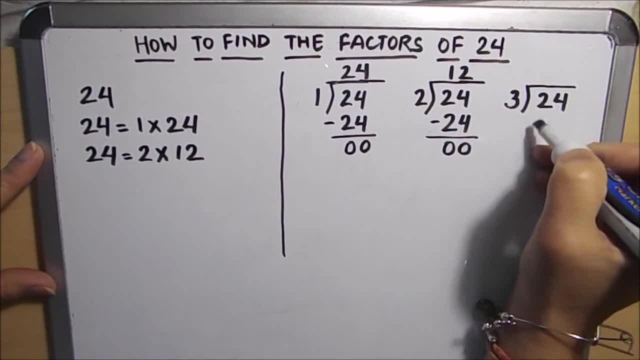 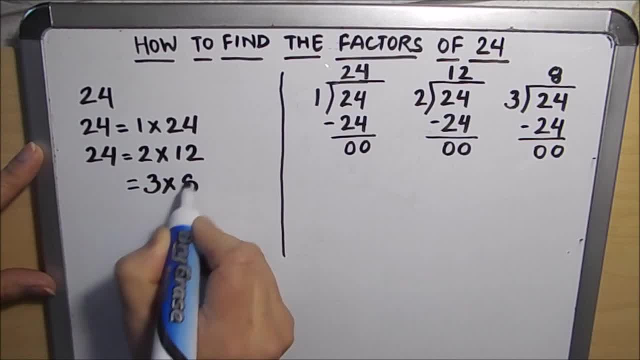 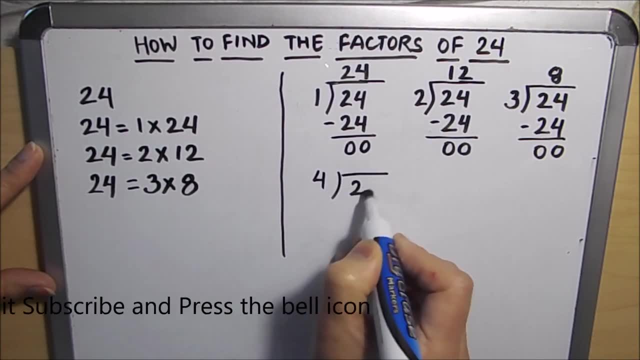 that 3 is also a factor of 24, because it is dividing 24 fully, without leaving a remainder. Next comes number 4.. Let's try and find out whether 4 is a factor of 24 or not. So we will divide 24 by 4 and we will count the tables and we see that 4 times 6 is 24.. So this is also dividing 24 and leaving 0. 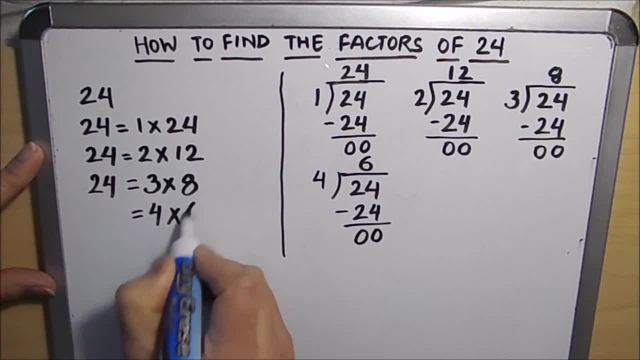 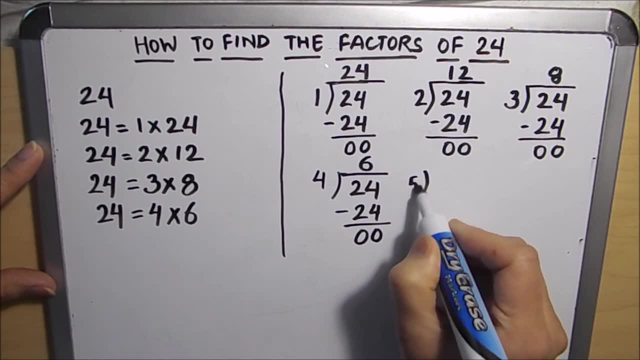 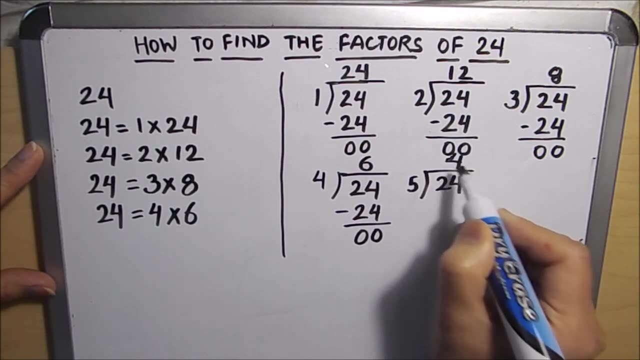 as remainder. So this proves that 4 is also a factor of 24.. Next we will move to number 5.. So we see that 5 times 4 is 20 and we are getting a remainder as 4 as a remainder. 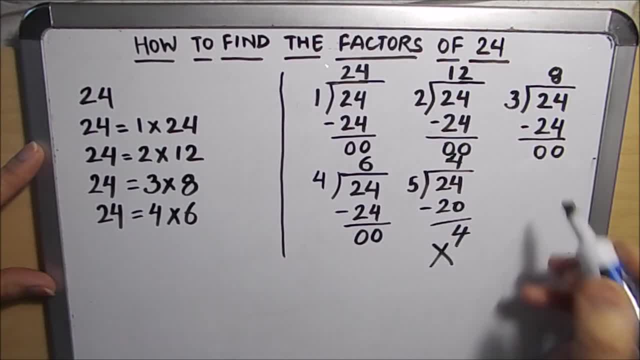 So 5 is not a factor of 24.. Next we will take number 6.. Now we see that 6 times 4 we have already taken. So here we see that this number is getting repeated 6 times 4 and 4 times 6. 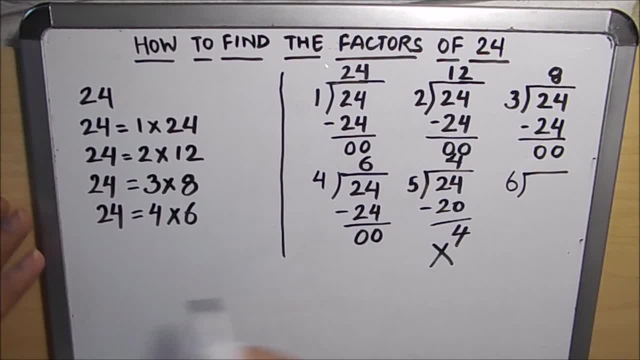 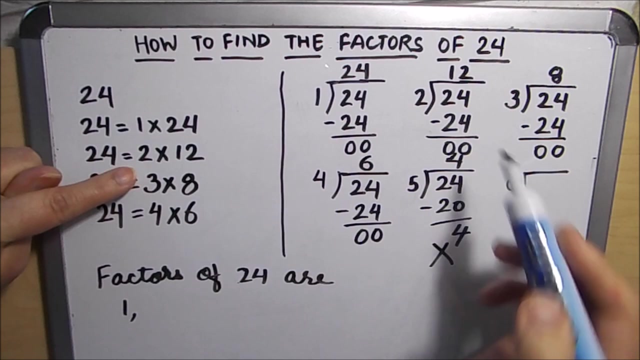 are the same thing. So we will stop here and then we will write factors of 24, as 1 is a factor of 24, as we have already seen here. So we will write 1 as a factor. 2 is also a factor. 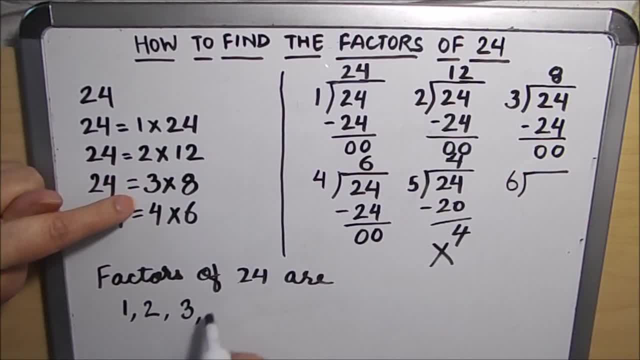 of 24.. 3- the next number is 4.. 6 is a factor of 24.. 7,, 8,. 7 is not a factor of 24.. 8 is a factor of 24, because 8 times 3 is 24.. So we will write 1 as a factor of 24.. So we will stop here and then. 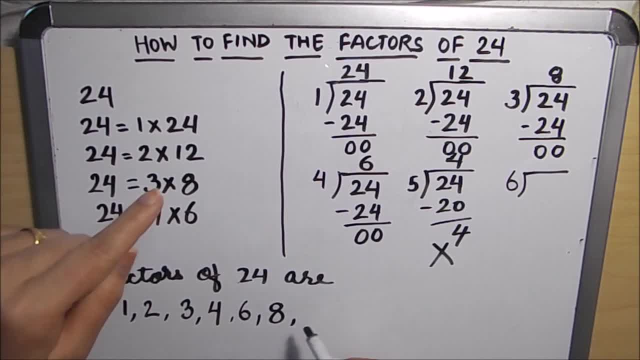 8 is there. Now, 12 is also a factor of 24, because 12 times 2 is 24 and 24, the number itself, is a factor of 24.. So this, these are all the factors of 24, and this is how we find the factors of any. 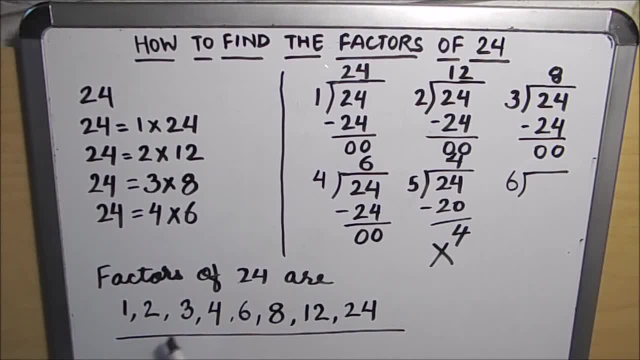 number. So the factors of 24 are 1,, 2,, 3,, 4,, 6,, 8,, 12 and so on. So we will write 7 as a factor of 24. this is how this is the process, by dividing the number by different numbers. 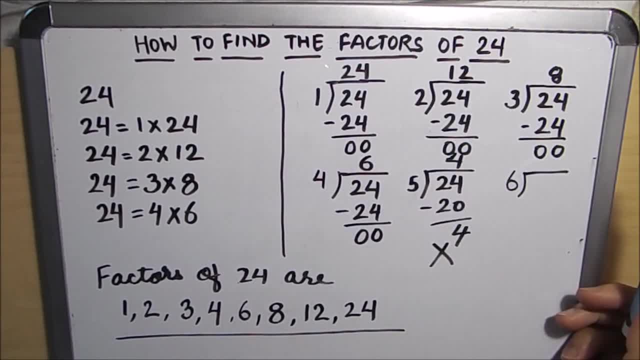 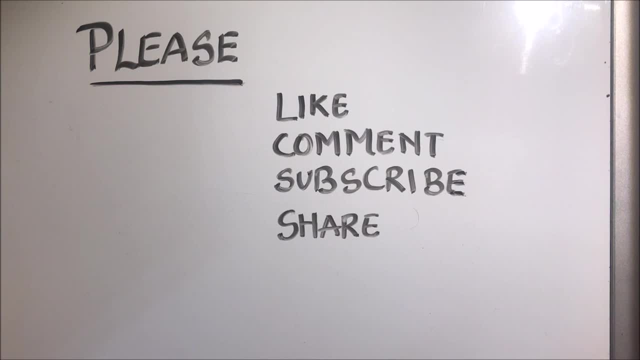 we can find the factors of any number. this is how you find the factors of 24. thanks for watching. please like, comment, subscribe and share my videos. thanks for watching.